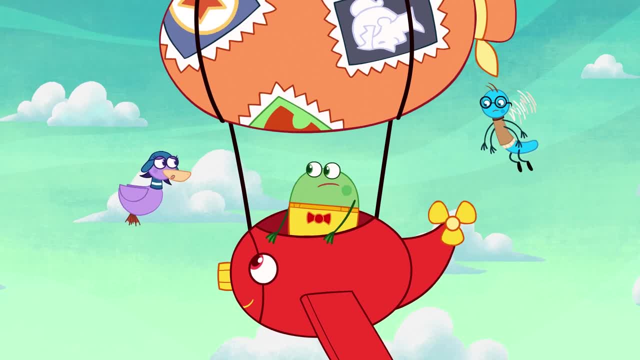 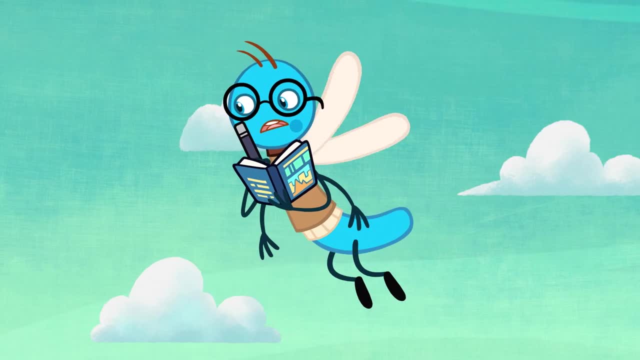 I don't know what's wrong with me. My luck just hasn't been so great lately. I'm not sure it's luck. that's the problem, Lorna. Come to think of it, all of our luck hasn't been all that good lately. 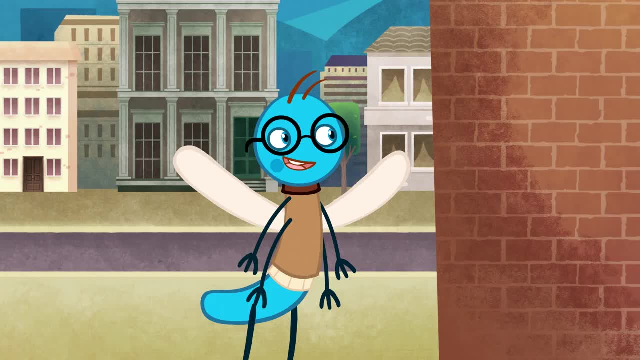 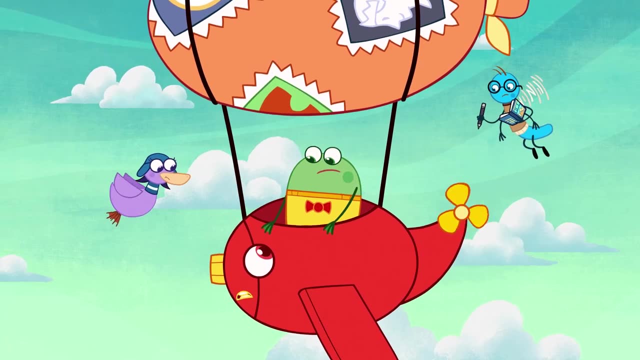 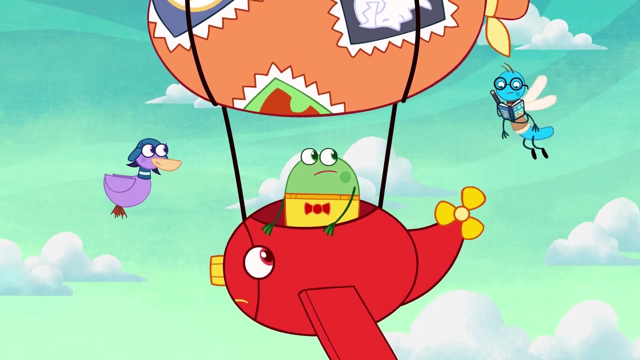 I've been keeping notes. All that bad luck. I wouldn't say it's bad luck, More like bad timing. And then my flying trick goes bad too. I'm going to add that to my list. Yep, there's no doubt about it. 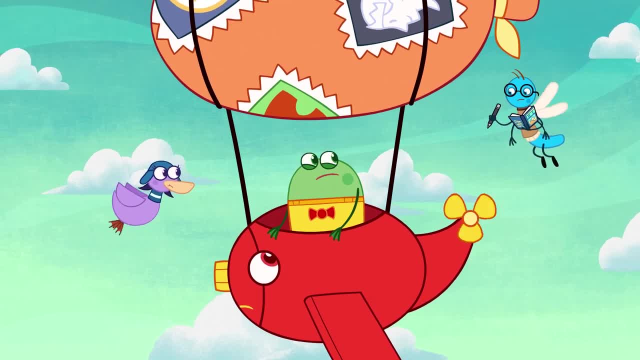 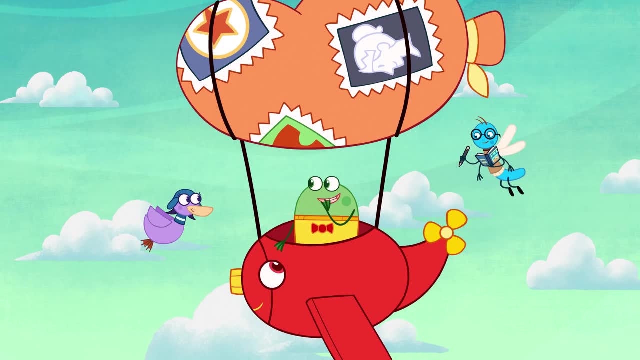 Sorry, Floaty, Our luck is officially bad. Okay, well, I give up. The good news is you're going to be happy about where we're heading today. Oh, that's right, I almost forgot. Today we're visiting Ireland. 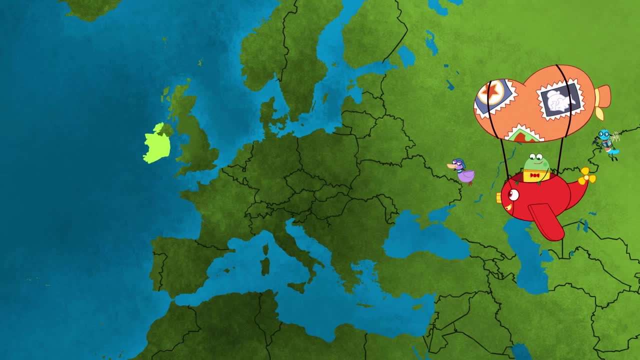 That's right, Hoagie. Ireland is a part of Europe, all the way over in the West, And it's so great they call it the Emerald Isle. A visit here is just what we need to know. Oh, that's right. A visit here is just what we need to know. 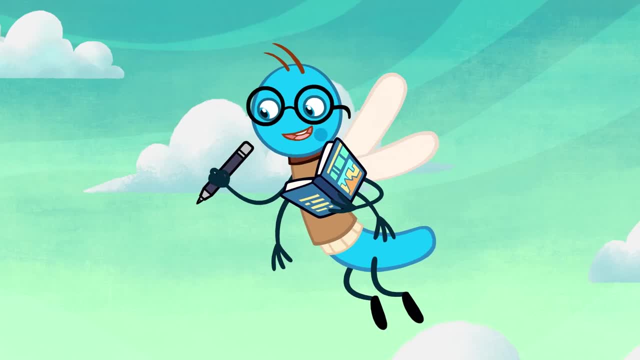 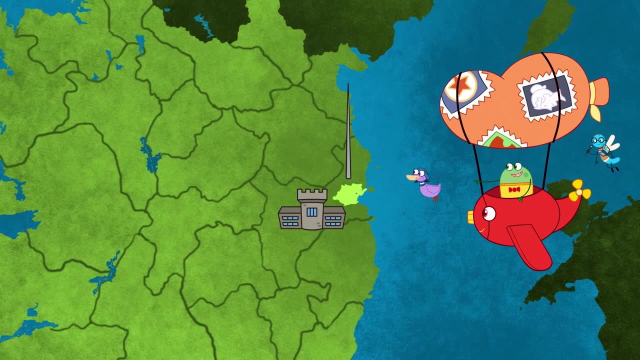 A visit here is just what we need to know. We need to get rid of our bad luck. Ireland is just about the luckiest place there is. Well, actually, I don't really believe him. Oh look, That must be Dublin. 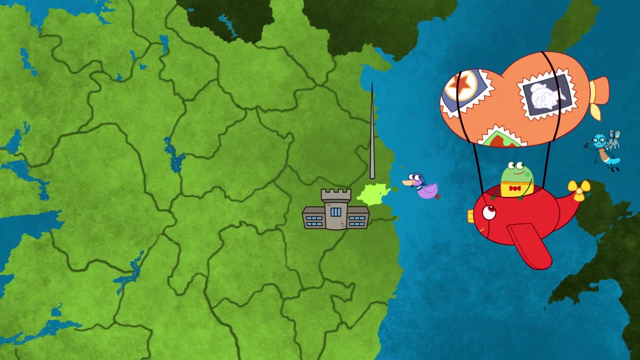 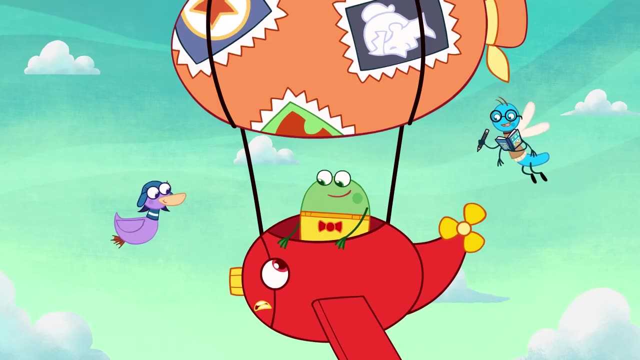 I love castles. They're all historical and stuff. Best of all, today is St Patrick's Day, the most important celebration in Ireland And um the luckiest day of the year. Awesome, Take us in for a landing Floaty. 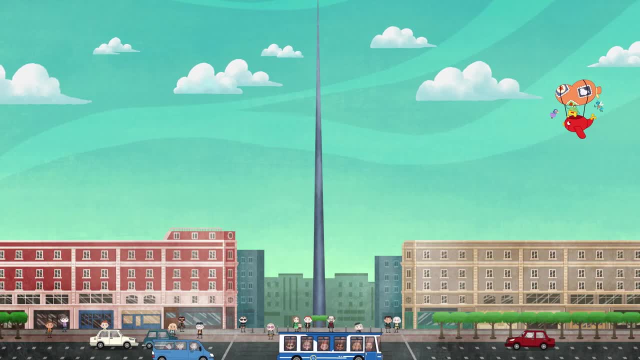 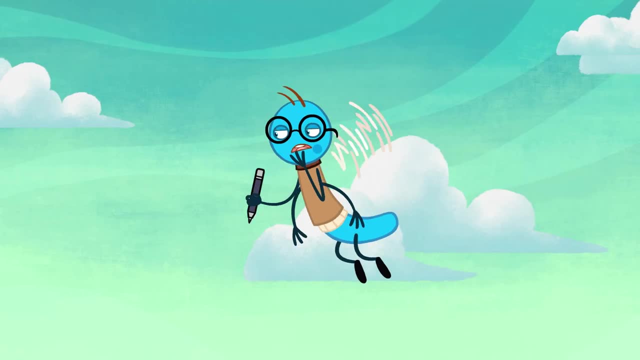 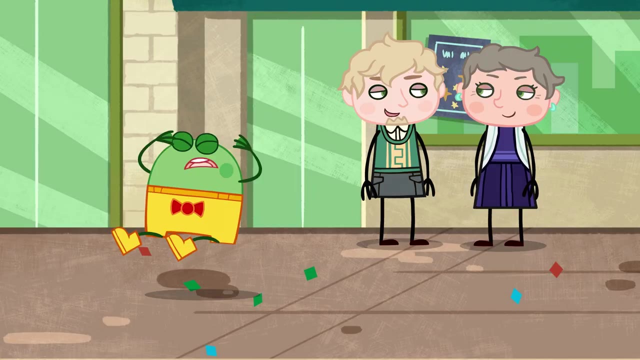 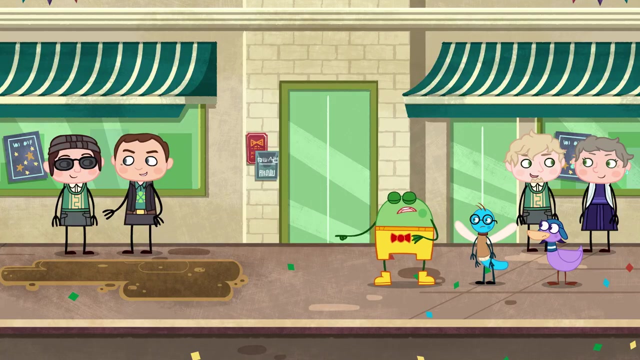 I think our luck is about to change. As long as we don't hit that giant needle, Because that would be bad. What needle? That needle? Don't panic guys, We just landed. It could have been worse. We could have landed in the mud, See. 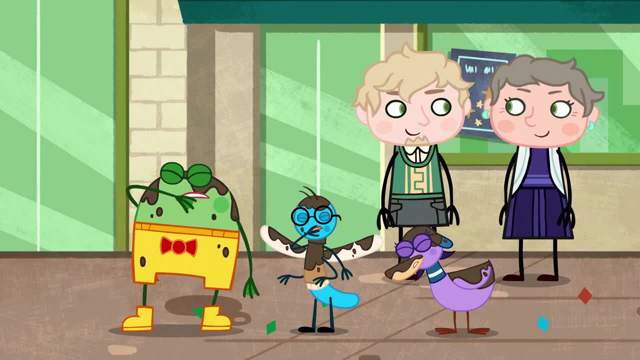 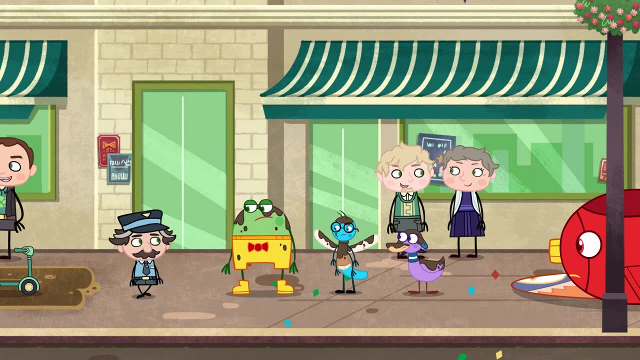 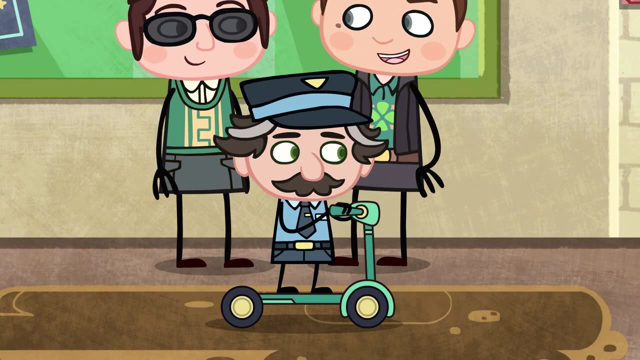 We just need to give the luck a little time to soak in Passport. please, Welcome to Ireland. May your troubles be as few and far apart as my grandmother's teeth. Did you see his Irish dancing? There was lots of jumping. 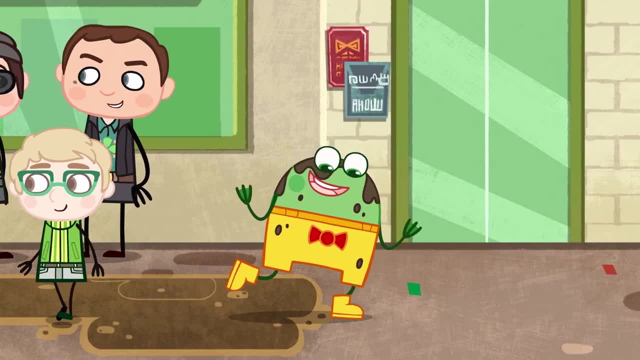 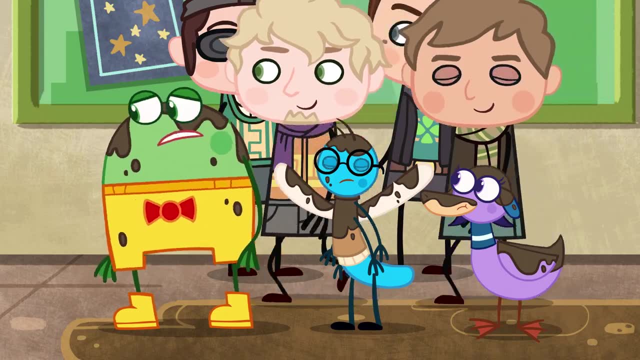 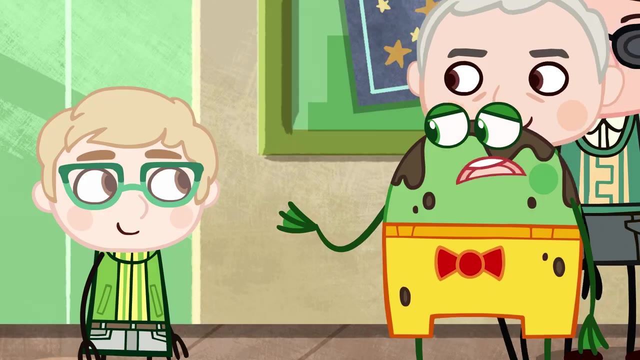 I'm great at jumping. I'm really sorry We've been having some bad luck lately. Bad luck You don't say Now, guys, We were hoping some of that luck of the Irish might rub off on us. Is that so? 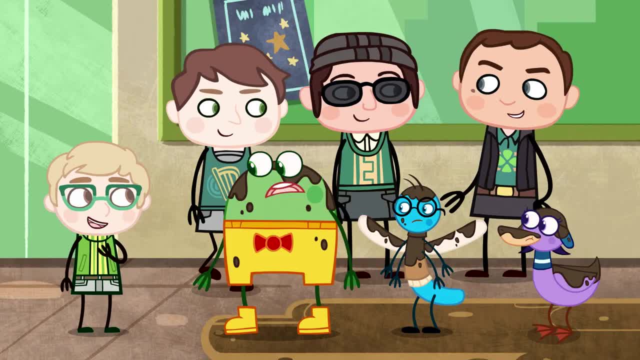 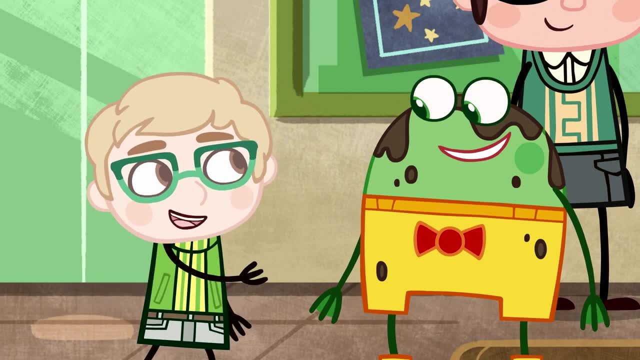 Well, I don't know much about changing luck, But I'm heading over to some of the St Patty's Day celebrations. if you'd like to join me, Yeah, Great. My name is Sean Patrick Connolly, Walsh O'Brien. Hi, Sean, My name's Hoagie. 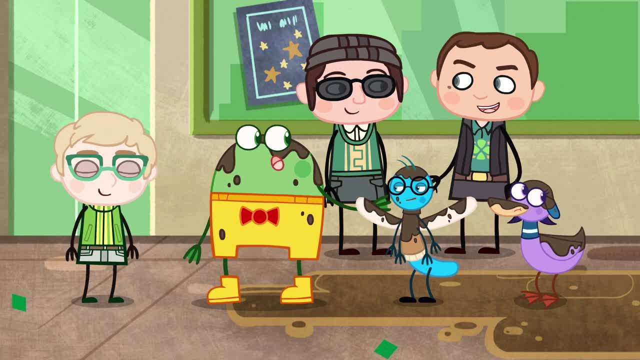 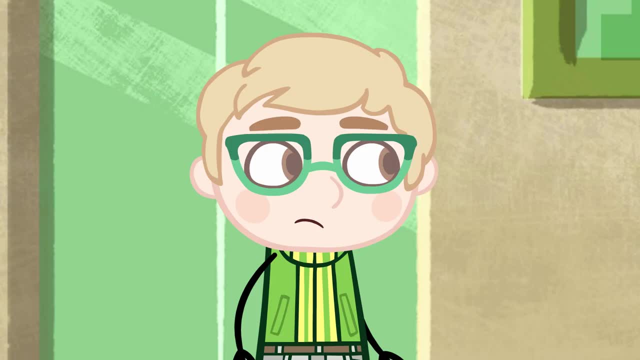 That's Bernie and that's Lorna, And this uh, not-so-floaty guy is Floaty. I'm usually much more impressive. I'm gonna have to find someplace around here to get my balloon fixed. Well, there's a tailor just at the other end of O'Connell Street. 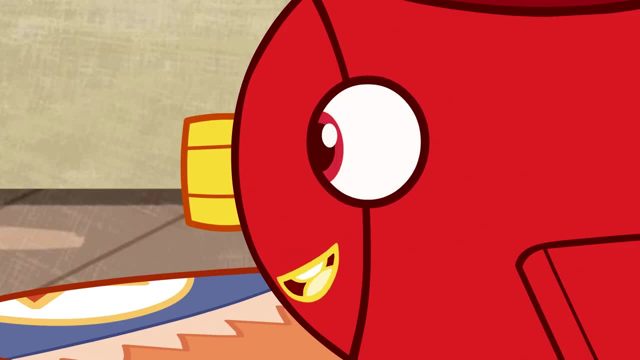 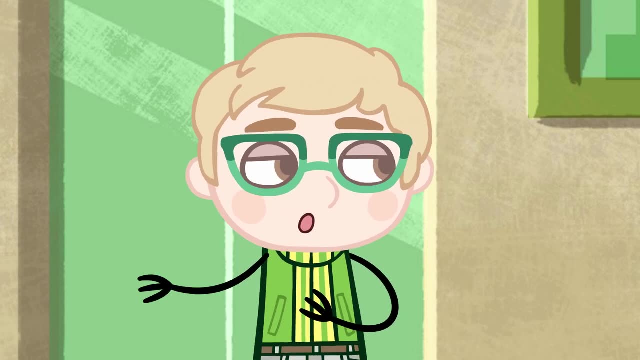 I'm sure he would be happy to patch you up. Thank you, That's a great idea. While I do that, why don't the rest of you look around Dublin a bit? Sure, It'd be my pleasure to show you around. 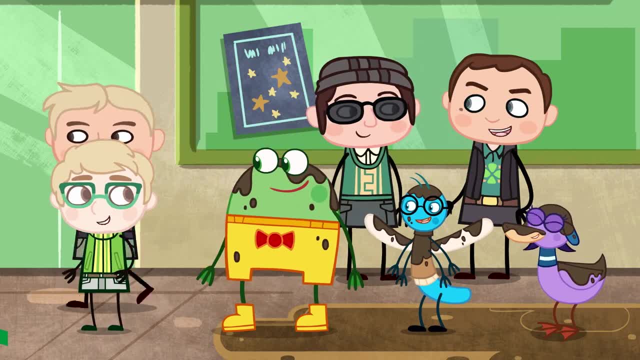 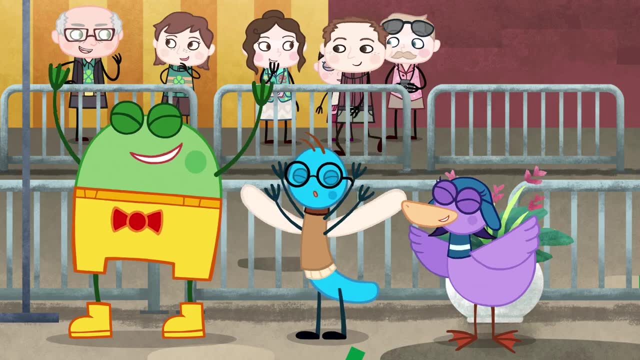 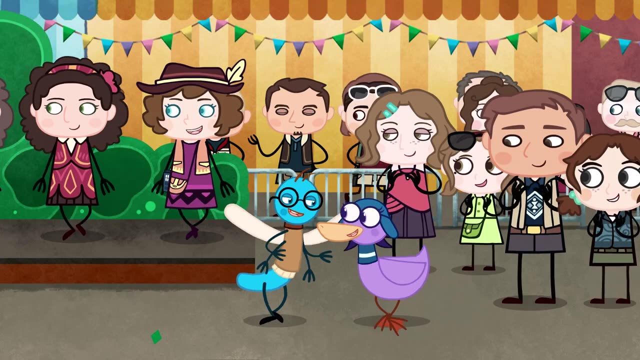 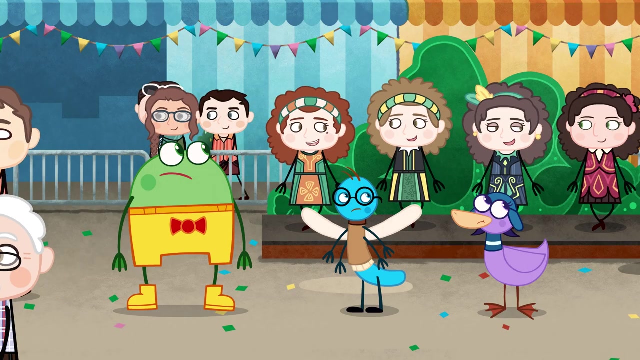 Yeah, Okay. Well then come on, Let's go see Dublin. How about a little dancing? Ooh, America Clues or St Patrick's Day Irish Folk Dance Festival. See you next year, everyone. Aw, it's over already. So much for changing our luck. 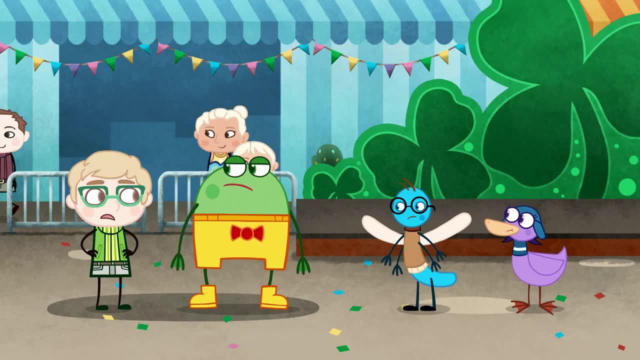 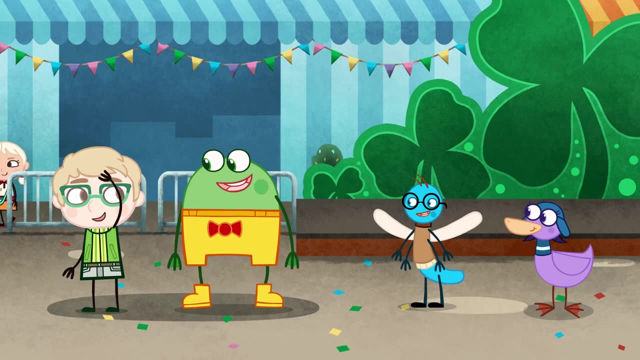 Hmm, I don't know about that. I think we're just late. I'm not ready to give up yet. Hmm, Let's see, Got it. Let's try the big St Patrick's Day parade. Come on, They're probably at Dublin Castle by now. 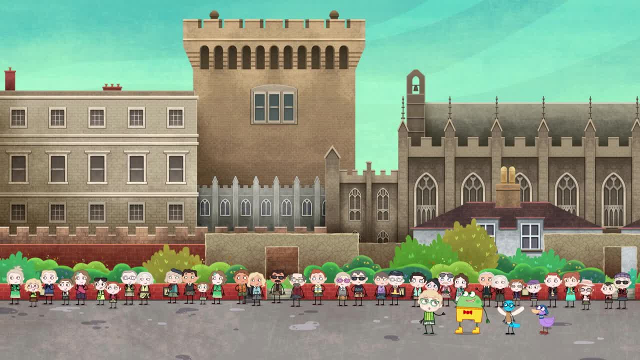 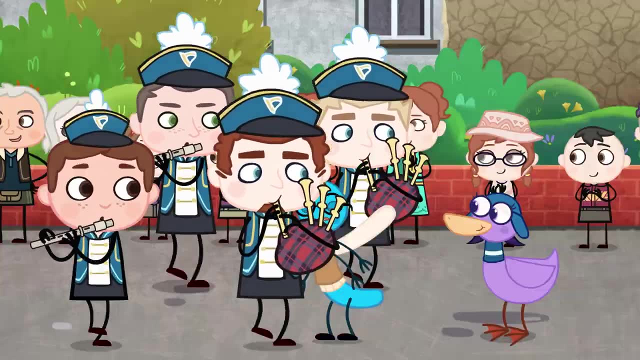 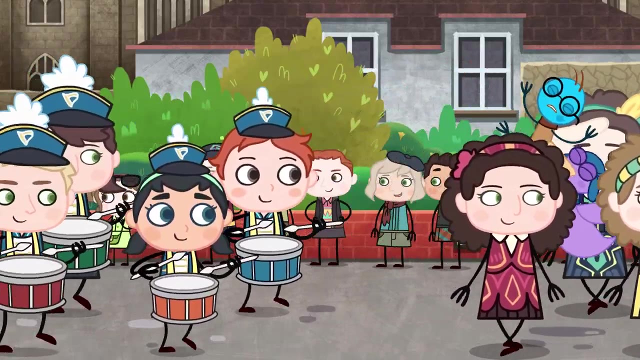 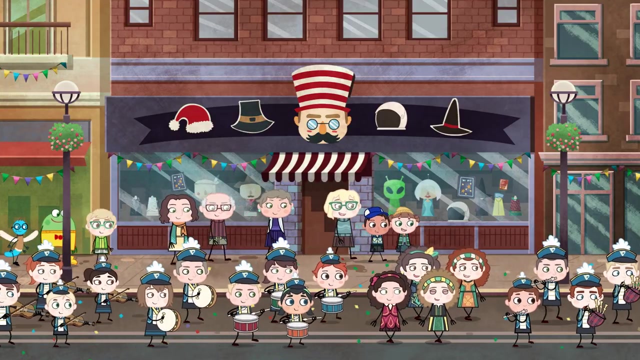 Oh, Is that a real castle? It sure is. Where's the parade? Sorry, Oh, excuse me, Sorry, I think we found it. We sure did. Yay, Woohoo, This is great, Oh, look. 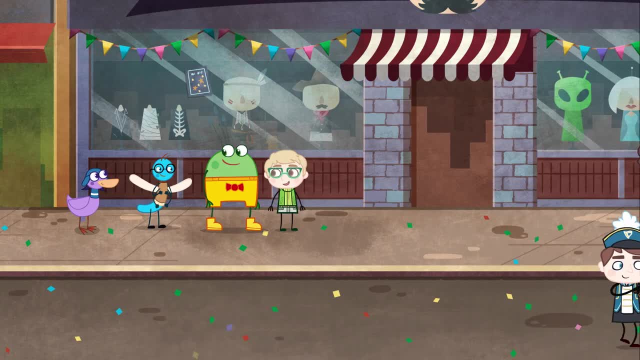 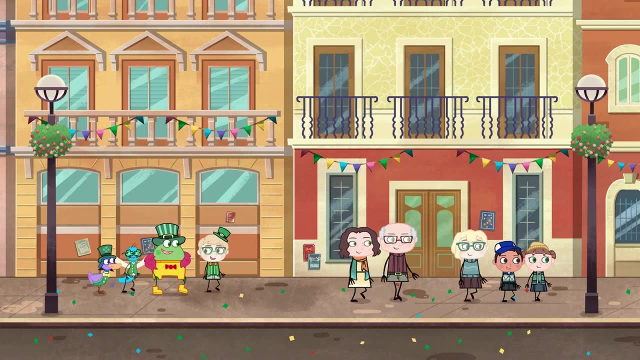 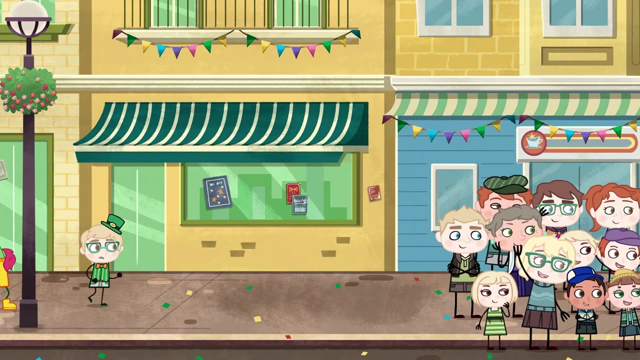 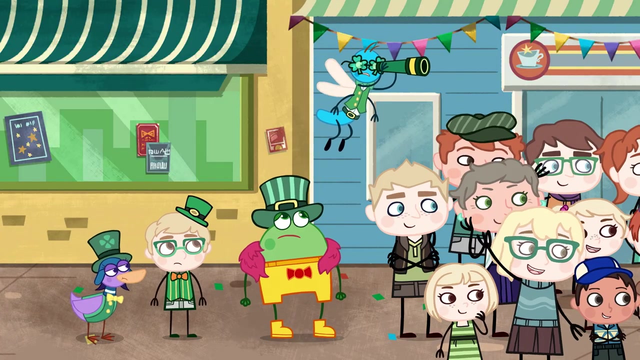 Yay, Let's get costumes. Great idea. Hey, Where'd the parade go? It's past us. It's way up in front now. Well, come on, then Let's go. Ugh, Ugh, It's no use, Hoagie, There's no room anywhere. 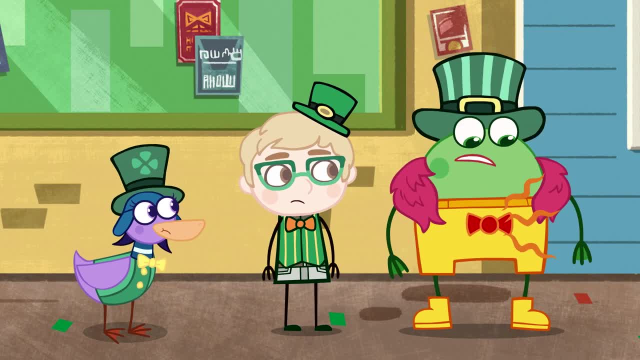 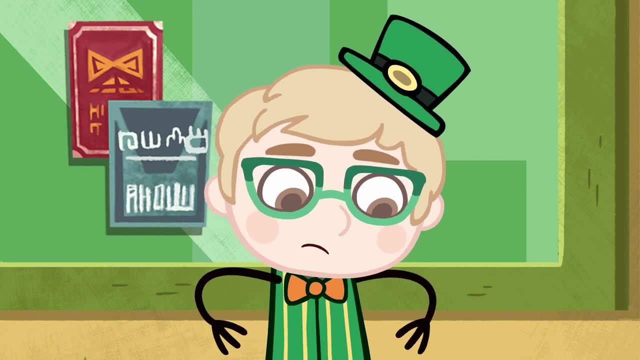 Ugh, Bad luck again. Huh, I don't know about that, Hoagie, Sounds like a thunderstorm is coming. We'd get soaked if we're in the parade in the rain. Oops, Sorry about that, It's not thunder. 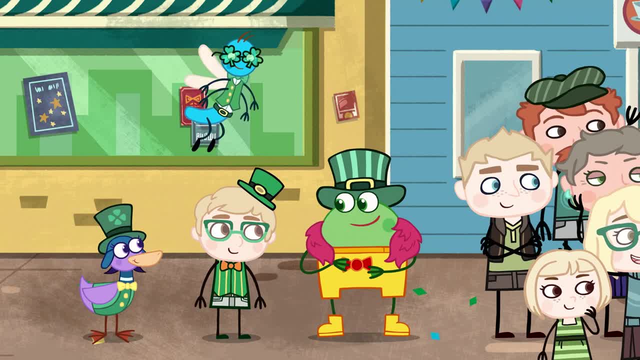 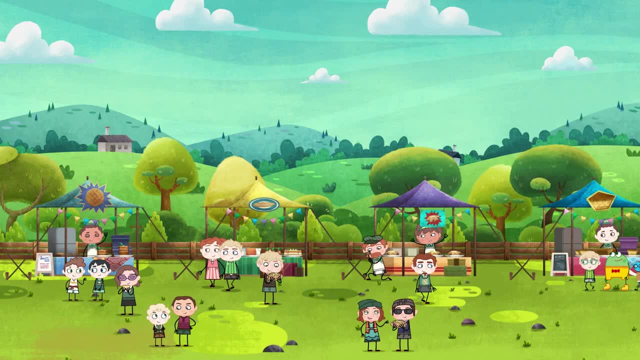 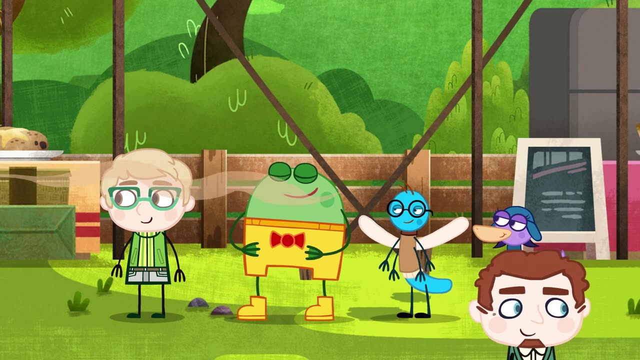 I guess I'm getting a little hungry. Then let's get something to eat. Yay, A full belly is a happy belly. My ma always says I like the sound of that. An outdoor food fair. Ooh, All that food smells so good. 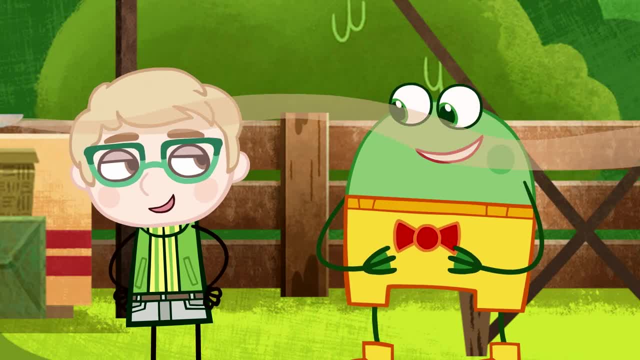 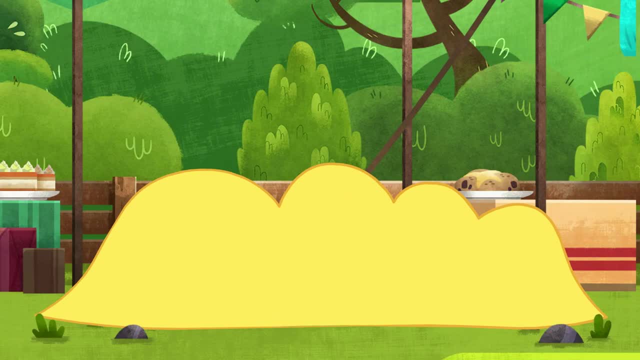 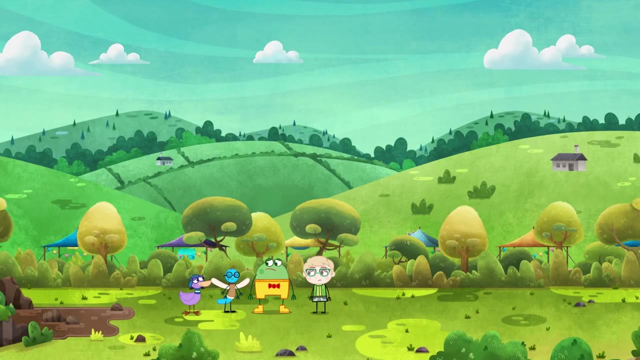 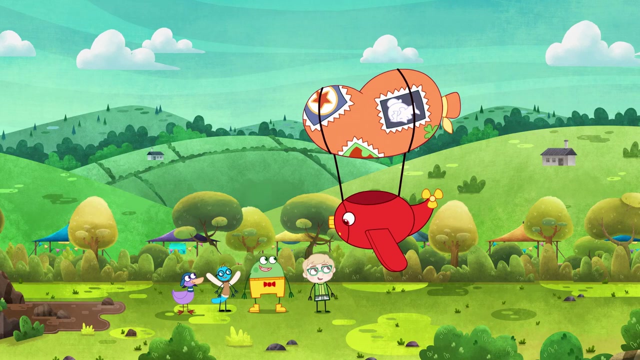 Finally a little luck. Then what are we waiting for? Ugh, Hey, I'm so sorry, sir. Well, that didn't go how I thought it would. Even more bad luck, Hello everyone. Look, Loni, You're all fixed. 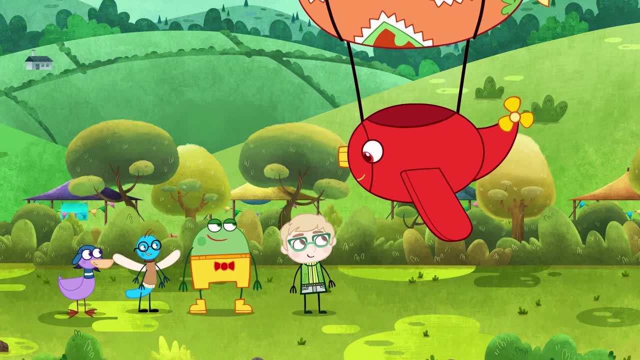 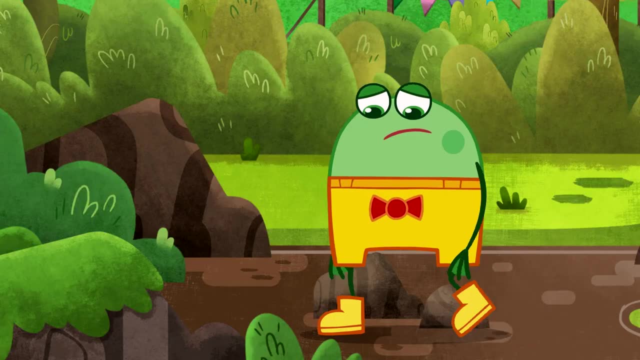 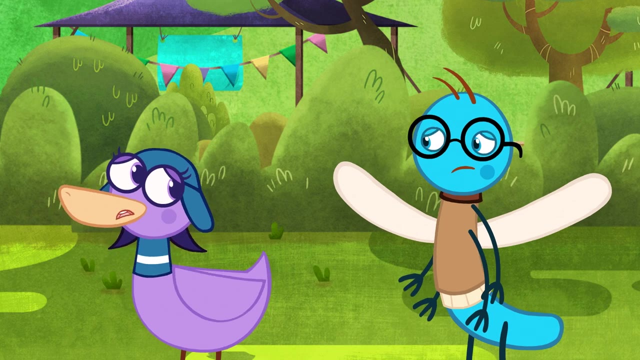 You look great. What are you up to? Well, we were going to eat something. He doesn't want to talk about it. Yeah, I'm thinking maybe our luck hasn't changed. I'm with you there, Bernie. Luck's all about how you 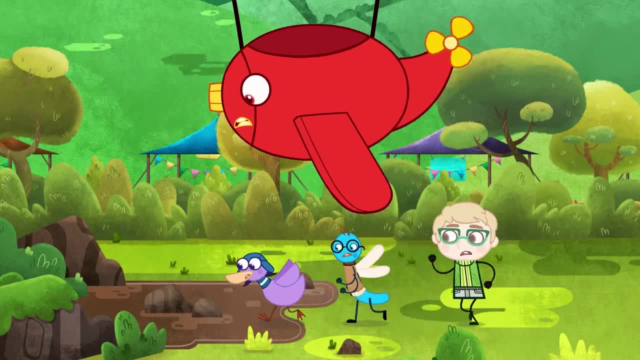 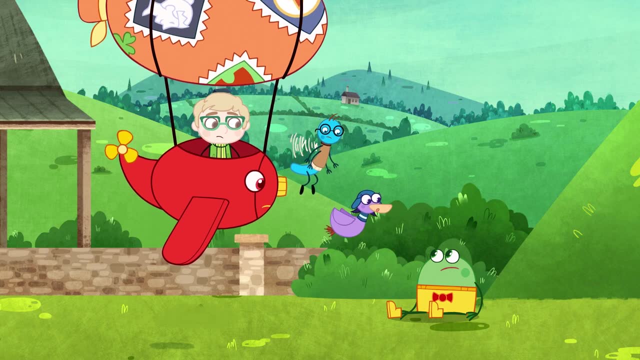 Ooh, be careful, Hoagie. I think it's safe to go. I think it's safe to say: our luck didn't get any better in Ireland after all. Yeah, In fact, I'm not sure it could get any worse. 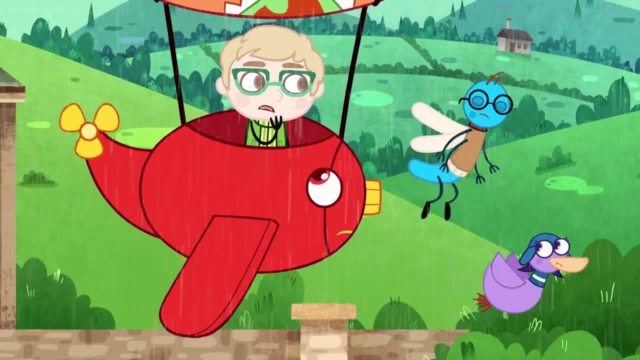 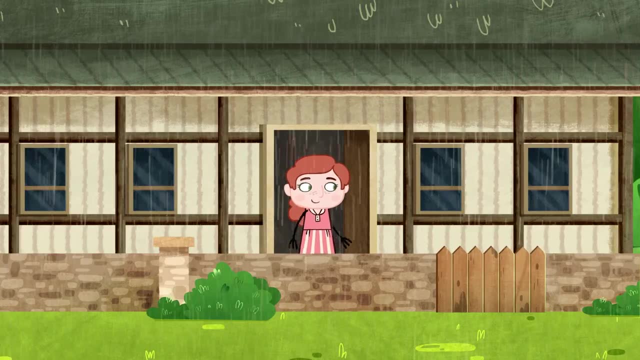 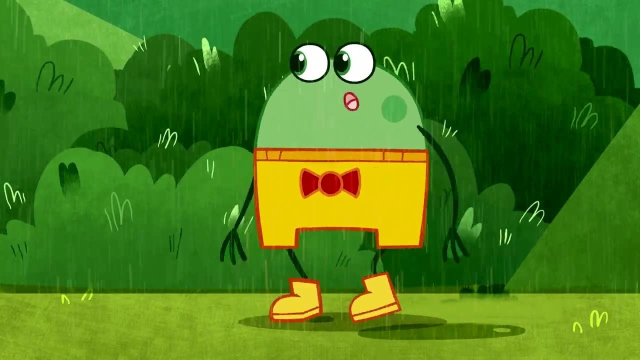 Huh Huh. Wait a minute. Maybe our luck has changed Really. I know this slope And that house, Sean Patrick Connolly Walsh O'Brien. I was just about to come looking for you, Sean. this is your house. 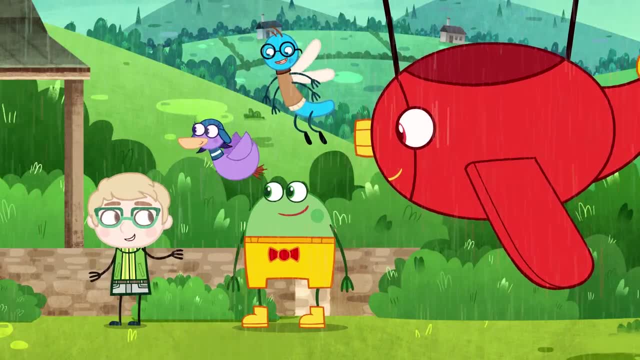 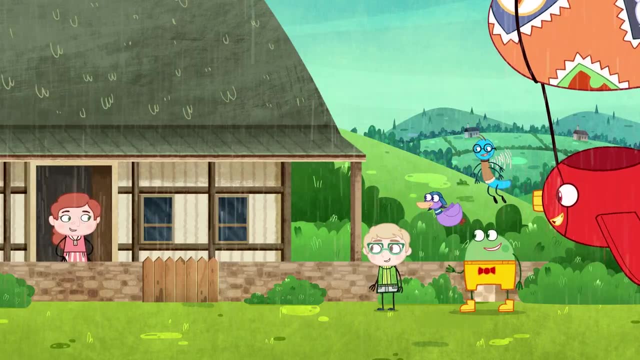 Of course it is. These are my new friends: Hoagie, Lorna, Bernie and that's Floaty. Hello Well, nice to meet you, But will you all be coming out of that rain and into the house for our St Patrick's Day celebration? 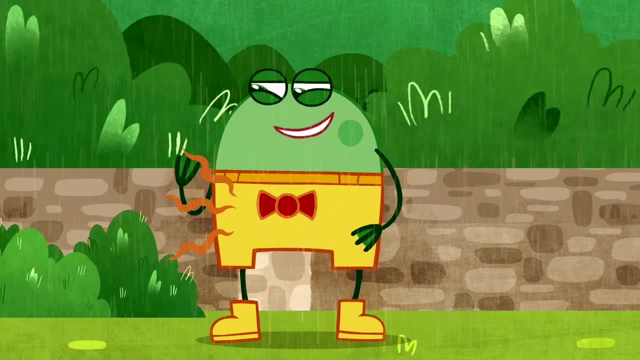 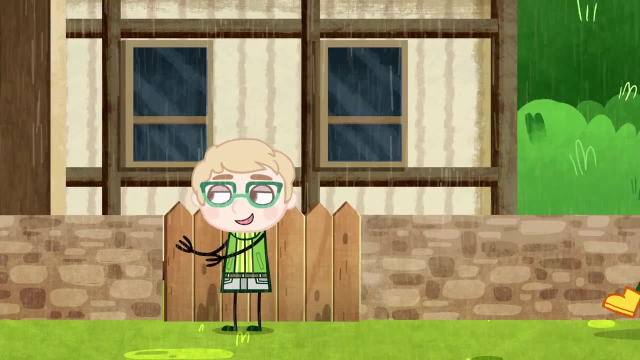 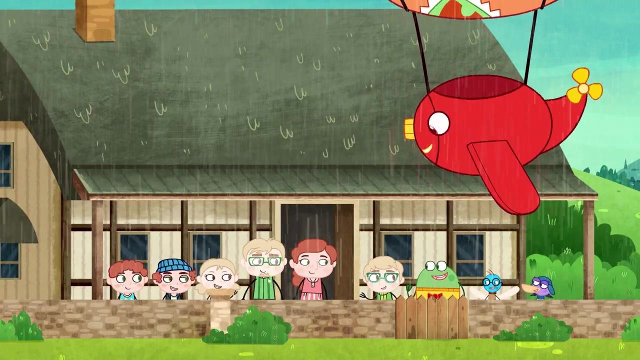 We've got plenty of food, So sorry, I'll take that as a yes. Yay, Hoagie, Lorna, Floaty, Bernie, I'd like you to meet my family. Hi, Hi there, Nice to meet you. 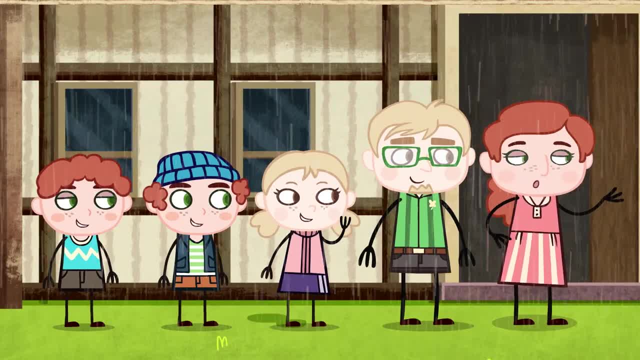 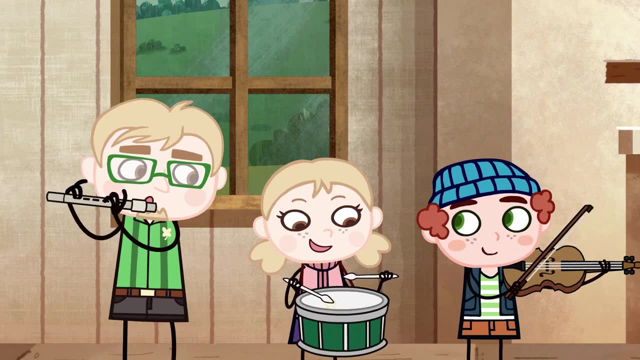 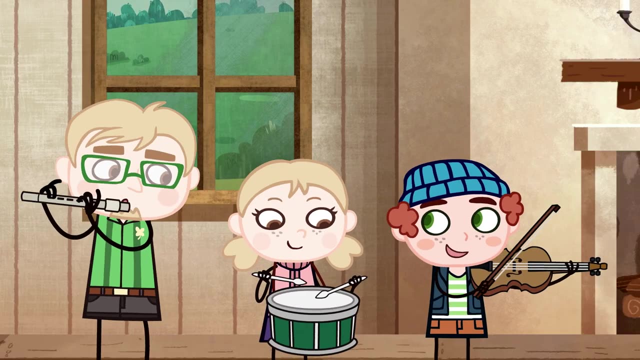 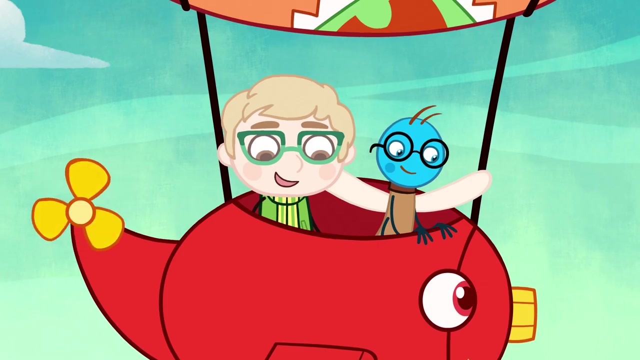 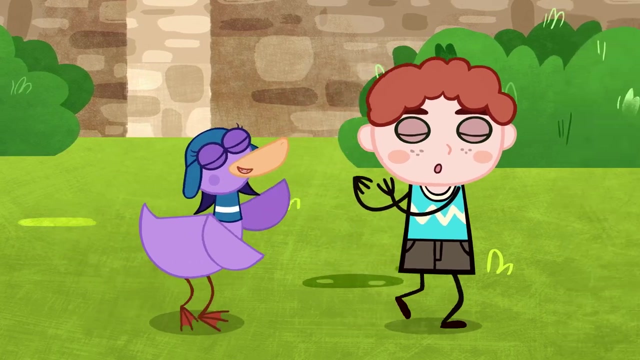 Nice to meet you. We like to celebrate St Patrick's Day as a family, but you're welcome to join in the fun too. Let's do it. Hooray time. Follow me, Hooray. I like this parade a lot better. 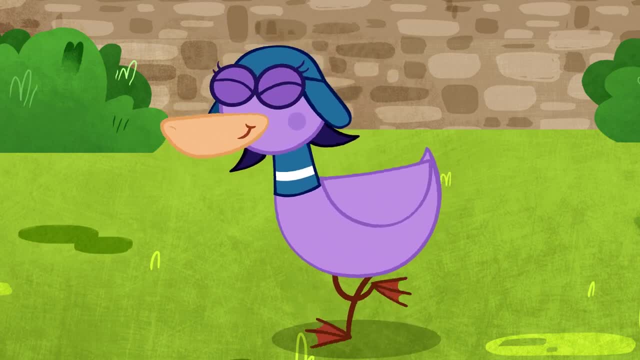 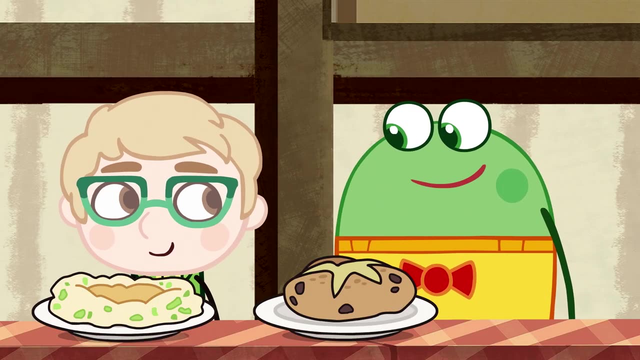 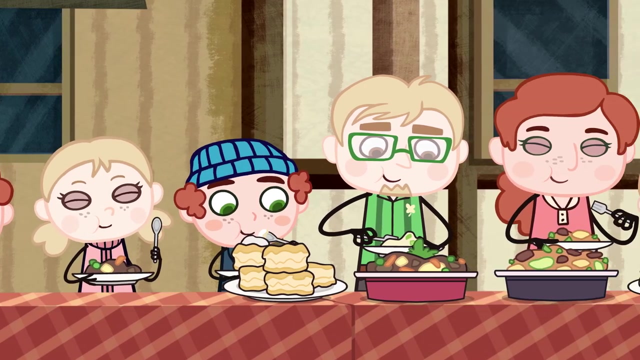 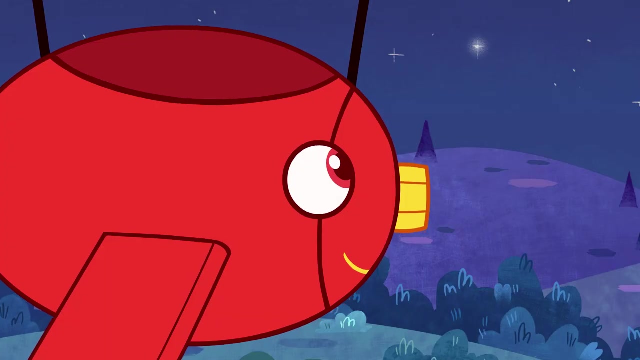 Yes, this is my kind of dancing. Ooh, That food looks so good. Dig in everyone. A full belly is a happy belly. I told you So, guys. I'm curious: Looking back, would you say today was a lucky day or an unlucky day? 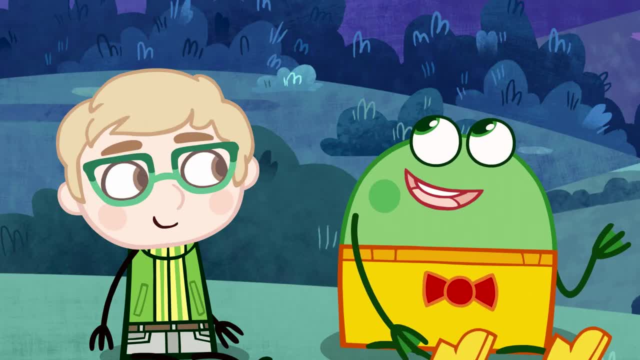 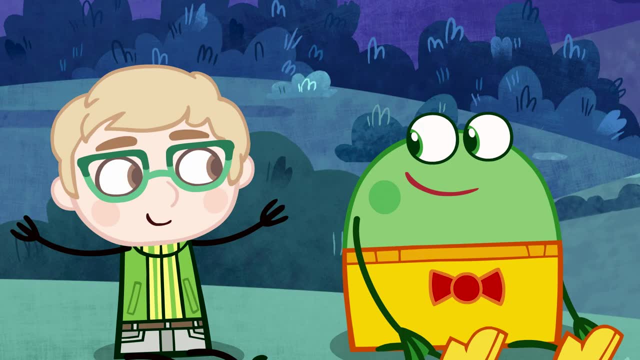 Well, it all started with me tripping and falling into Sean and knocking him down. True, But if you hadn't knocked me over, we might never have met at all. And if we hadn't knocked him down, debate's on hadn't met you, we'd never have tumbled down the hill and we wouldn't have ended up at 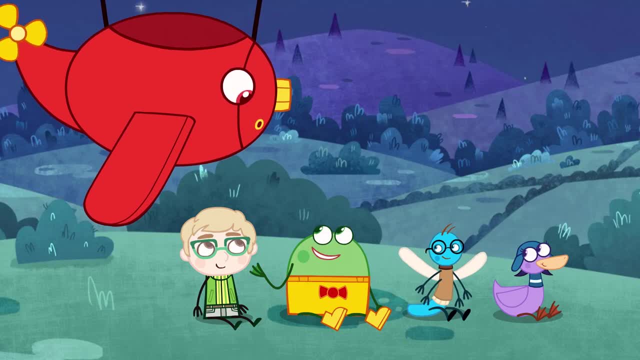 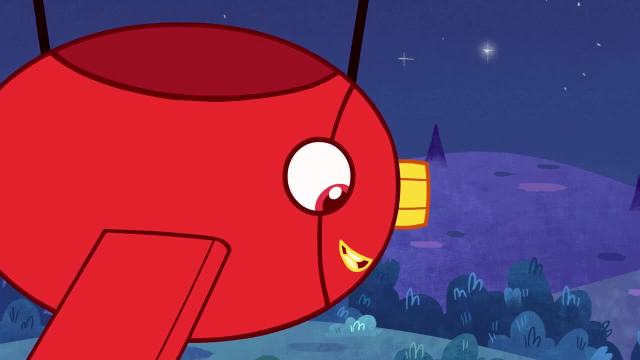 your house and met your awesome family. So, So yeah, now that I think about it, this was a very lucky day. You see, That's what I was trying to tell you all day. Luck is all about how you look at things.